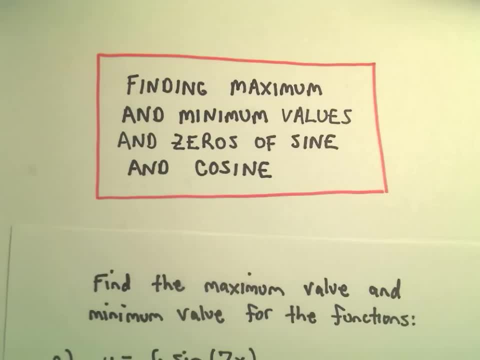 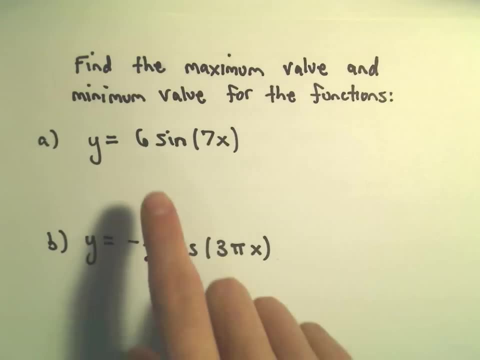 All right, in this video I just want to do a couple examples about finding the maximum and minimum values for different sine and cosine functions. And in this case we've got 6 sine of 7x and then negative 1 half cosine of 3 pi x. 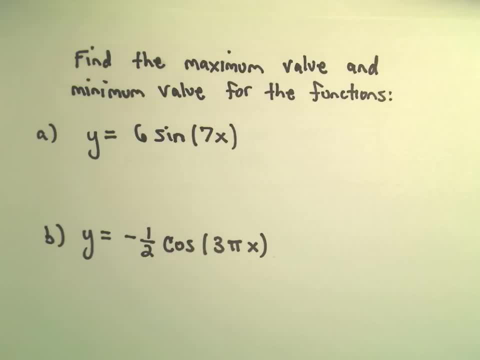 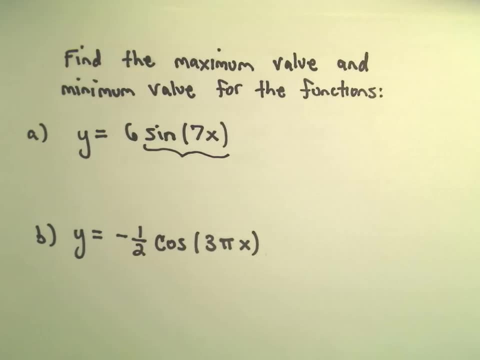 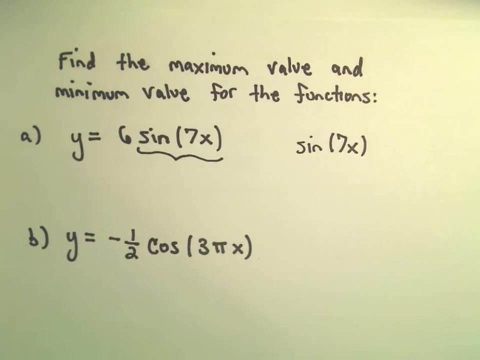 Okay, a couple different ways, I guess you can go about thinking about this. To me, you know, when I look at this, the first thing I see, for example, is the sine function, So sine. if you think about you know, if you think about the graph of it, you know a couple different arguments, I guess here. 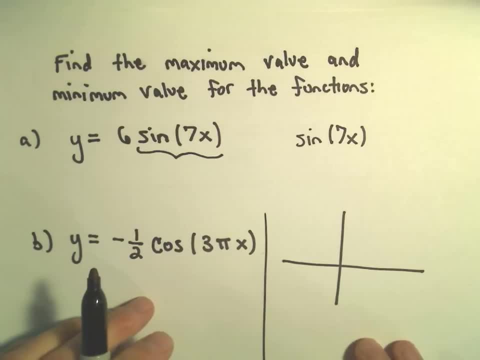 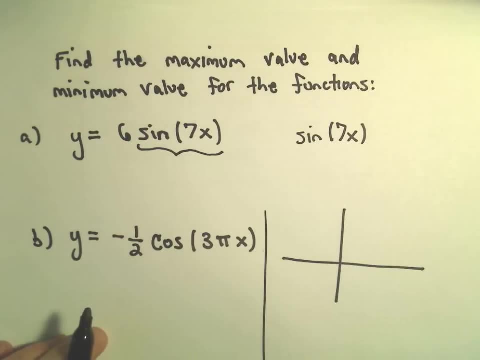 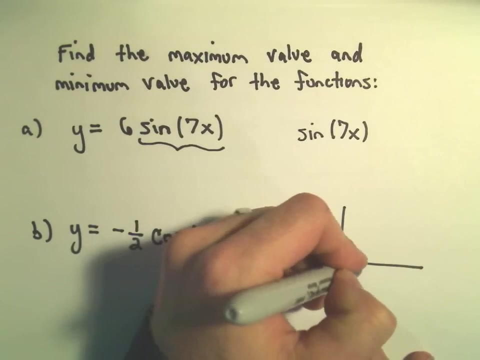 Remember, by multiplying by the 7, all that's really going to do is just change the period. So I'm forgetting about the 6 for a second here. All that's going to do is change the period. So, okay, maybe it's going to do things a little faster. 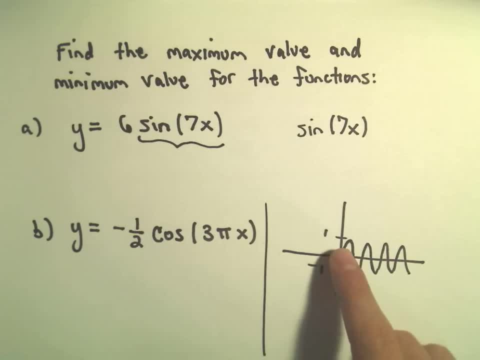 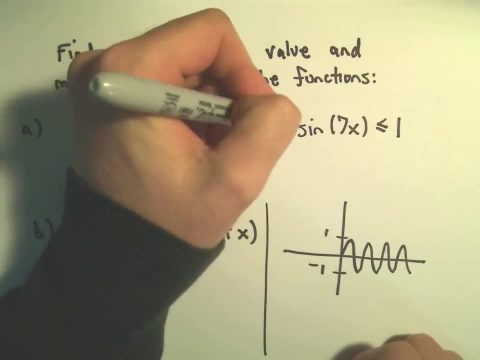 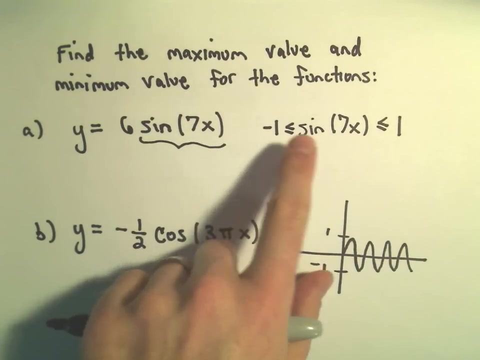 But still sine. the sine of some value is always between- is it most positive, 1 and the smallest it ever is is negative 1.. So really I'm just thinking about the range of 7 sine x. It's always between negative 1 and positive 1.. 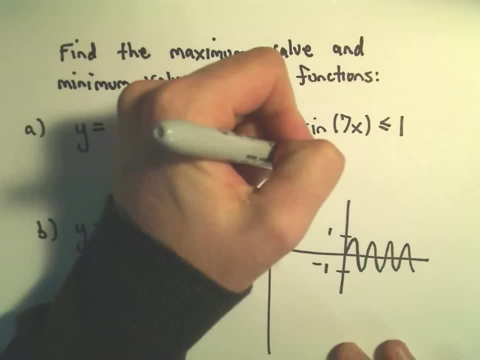 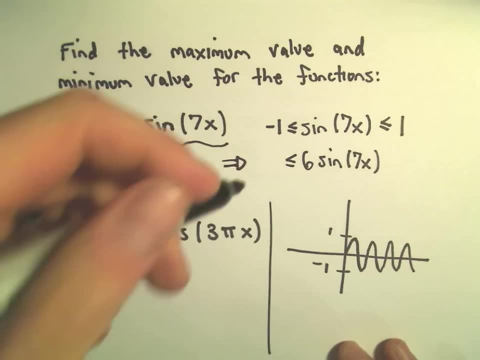 Well, what that means is if we multiply the inside by 6, so it says 6 sine of 7x. Well, I would have to multiply the inside by 6.. I would have to multiply the left side by 6 as well, which is negative 6.. 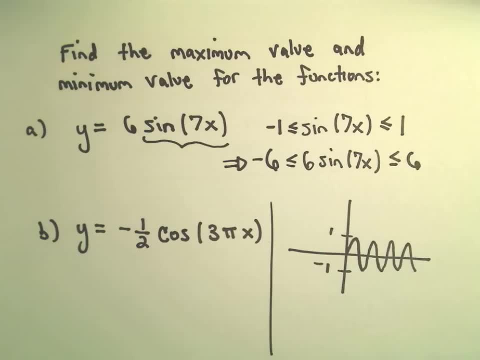 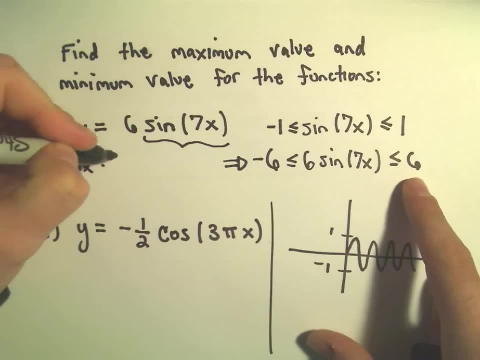 I would have to multiply the right side by 6 as well, which would give me positive 6.. And these are going to be your maximum and minimum values. The maximum value is going to be just 6.. And the minimum value again is going to be negative 6.. 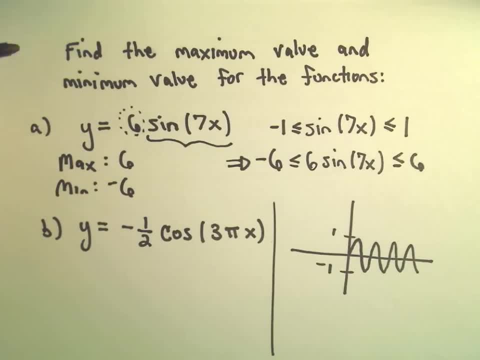 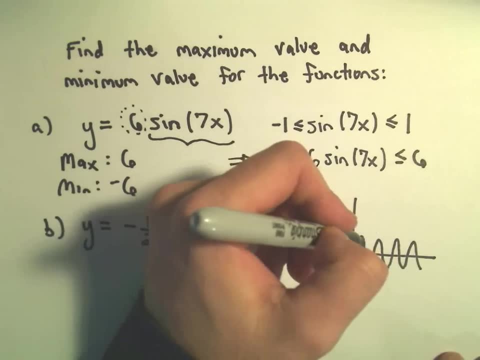 So, again, definitely taking this coefficient into account, kind of thinking about the amplitude here, how this coefficient changes the amplitude: Instead of being positive 1 and negative 1, it's now going to go up to 6 and negative 6 when we graph it. 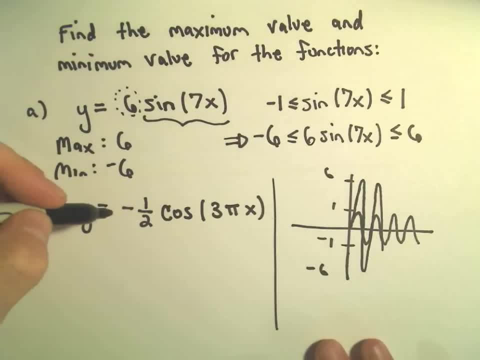 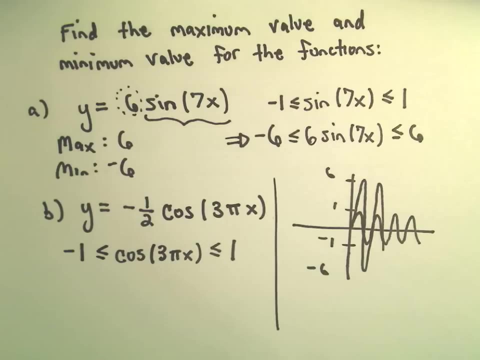 Okay, So the same thing for our next one here. negative 1 half times cosine of 3 pi x. Well, again the same argument. Cosine of anything is in between positive 1 and negative 1.. And again, notice, there's no restrictions on the domains.